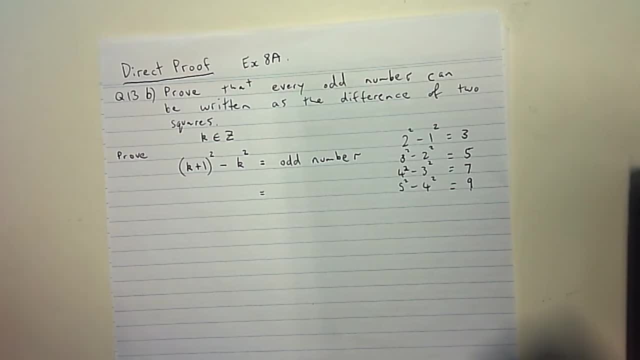 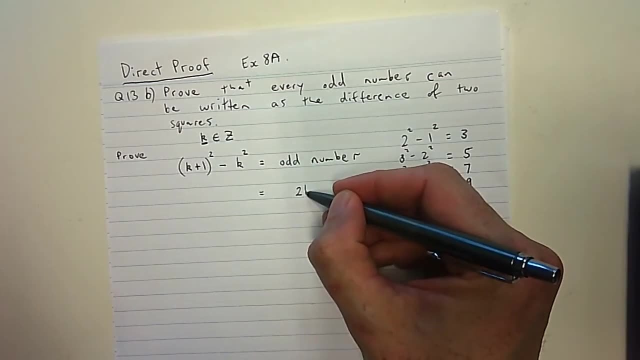 Okay, I could write an odd number. Let's start with an even number. That'll be easier first. Now, if I get any k value, any integer, and if I multiply it by two, no matter what that integer is, if you multiply it by two, you have an even number. 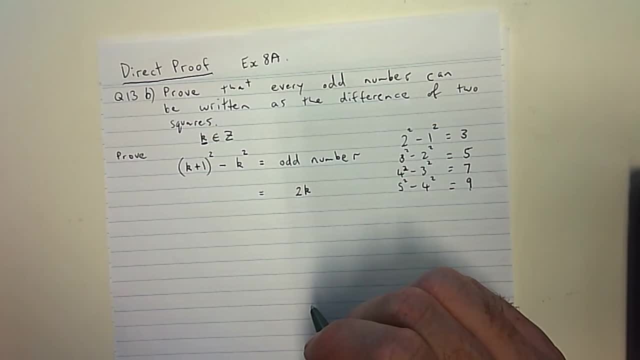 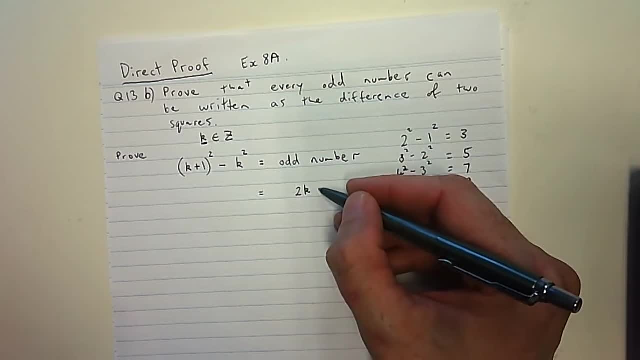 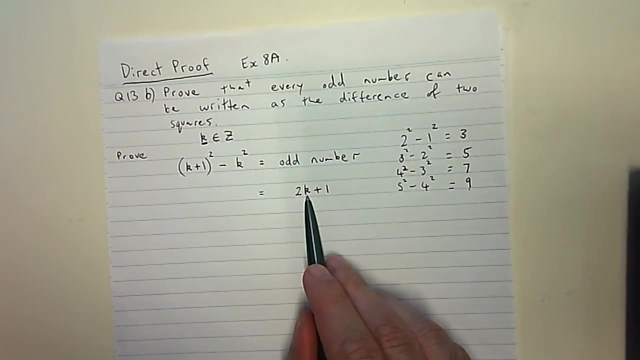 It's always going to be an even number if you multiply it by two. So to get an odd number, all we have to do is get this even number which we've created and add one to it. So you can say that if you've got some number, any integer, multiply it by two and add one. 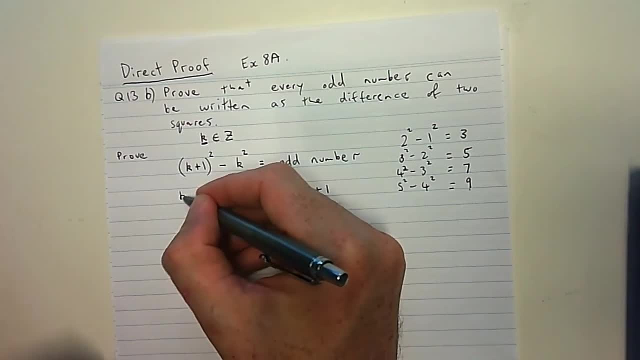 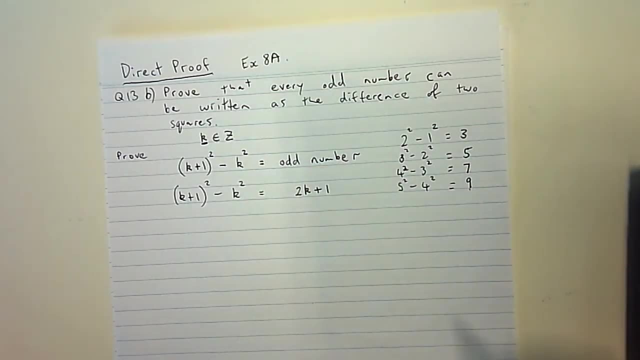 to it. it's going to be an odd number. So I'm going to say, basically, let's get k plus one squared. take away k squared and prove that that's going to equal two k plus one. Alright, so let's start with the left-hand side of this equation. 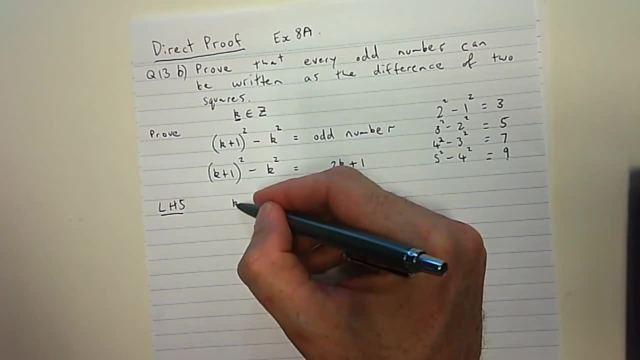 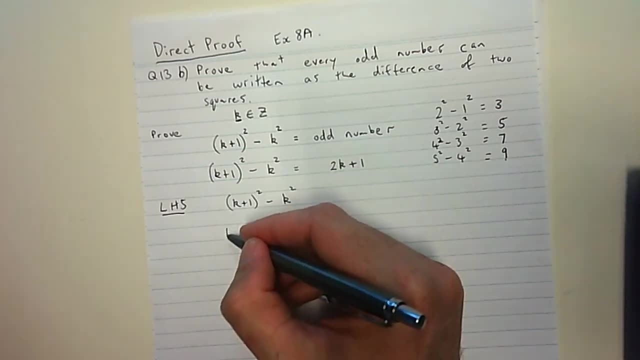 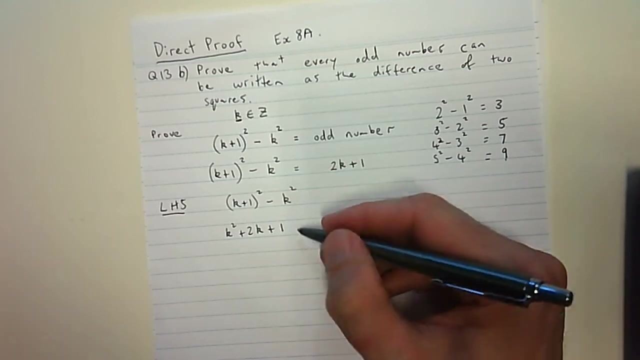 So I'll just write LHS over here And I'll get k plus 1 squared. take away k squared. So expand out the brackets to start off with, So that'll give us k squared plus 2k plus 1.. I'm taking away k squared from that. 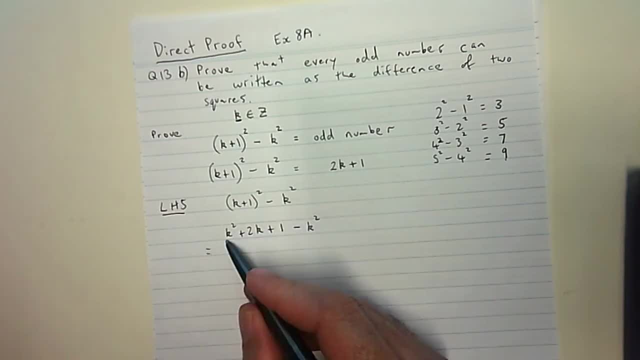 And then, once I've got that, if I have k squared and I take away the k squared, I'll be left with 2k plus 1.. Now we can say: therefore, left-hand side of this equation is equal to RHS. 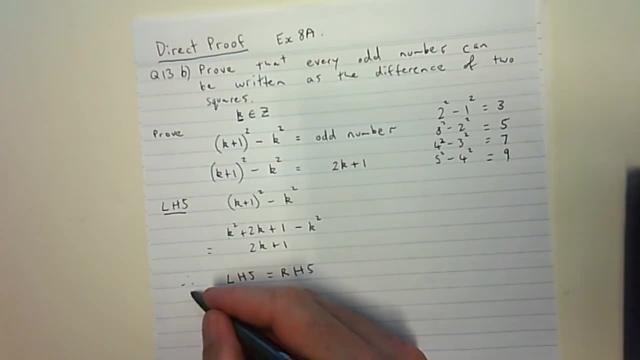 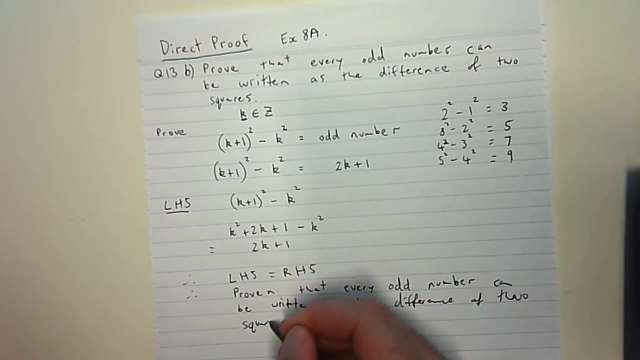 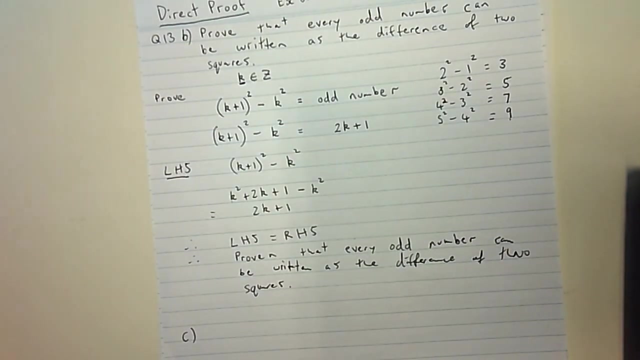 the right-hand side of the equation And I can say, therefore, proven, Proven, That every odd number can be written as the difference of two squares. Okay, so that was B. Question C then asked for: Hence: prove 101 as the difference of two squares.